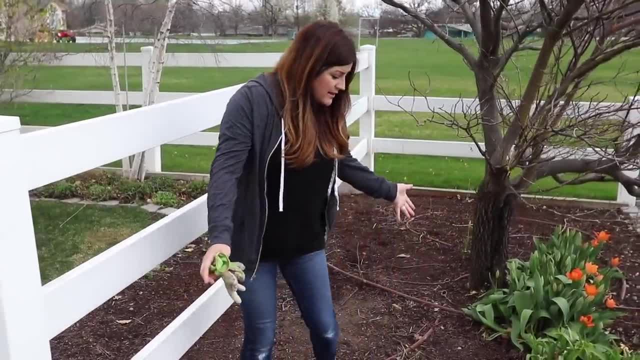 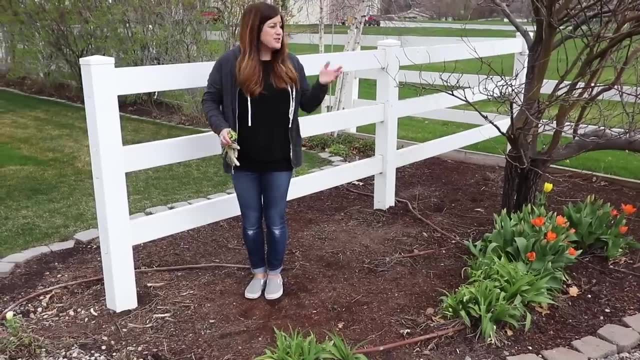 bloom color and your foliage. I'm going to have to add a little bit of water in here because I'm going to have to keep my foliage color. even in a small area like this- like maybe I'm dealing with eight feet, six feet and it's kind of an arc- I want to make sure that it's pretty all year round. 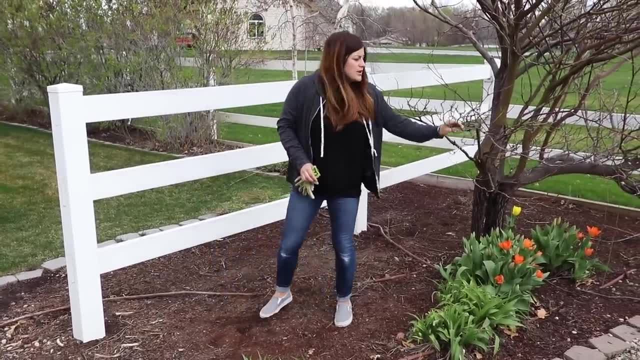 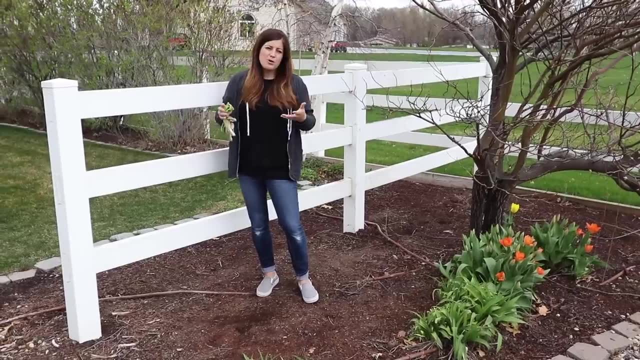 so I do have some winter interest going on. This is a pagoda dogwood tree, so it has green leaves. so, knowing that when I go in to choose my anchor piece right here, I'm going to go with something red, so that they contrast each other, so that they are set apart from each other, and also when I go 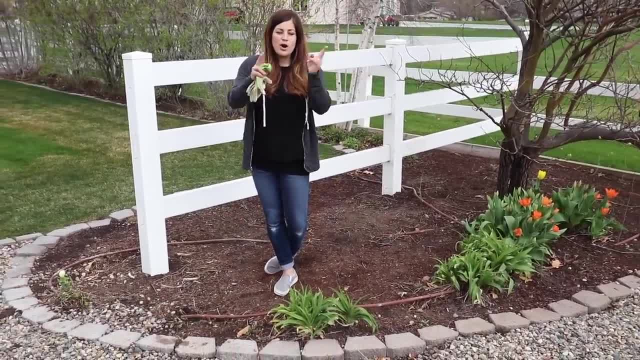 in with my perennials. here I've chosen two different kinds that will overlap very well with the colors, and then I'm going to go with some plants that are a little bit more natural. so I'm going to go with the ones that are a little bit more green and a little bit more red and a. 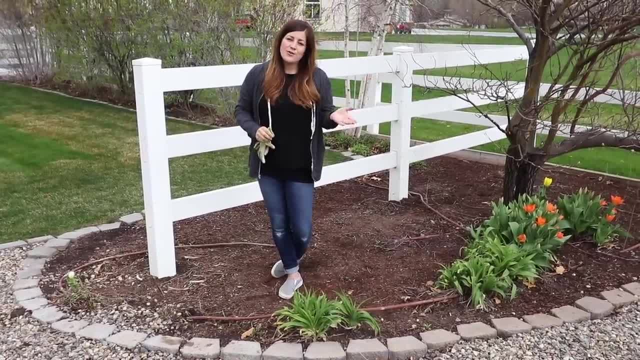 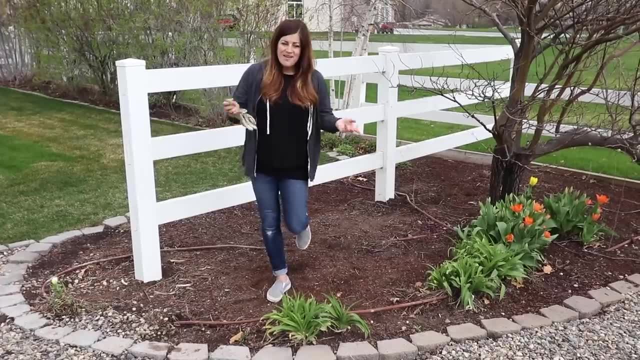 little bit more blue and a little bit more green. These plants bloom a little bit, but one starts late spring and goes to mid summer, and then the other one starts mid summer and goes through the rest of the season. so I make sure to have color all throughout the whole year and I think that's. 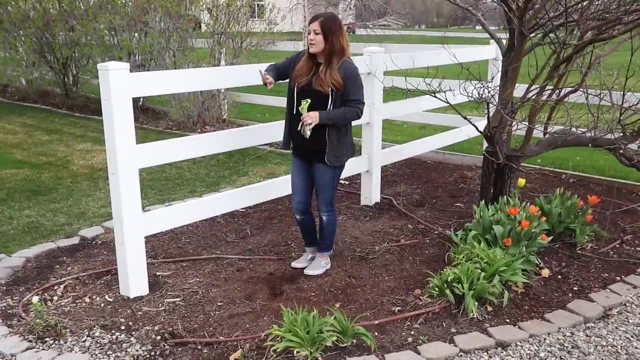 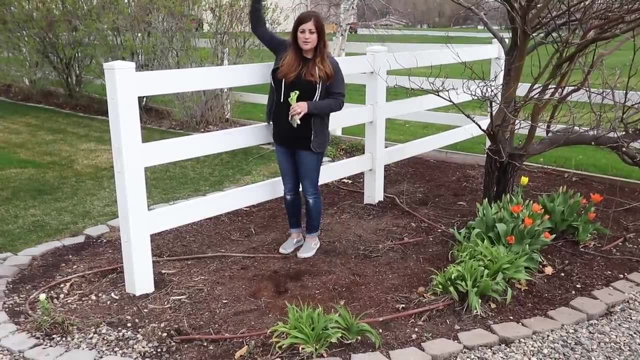 really important, so that you just have something beautiful and you can enjoy all the areas in your garden all the time. The last tip is to layer, So most flowerbeds have a natural back to them- they're first- and work your way down. that way you can see each plant individually. there's nothing blocking. 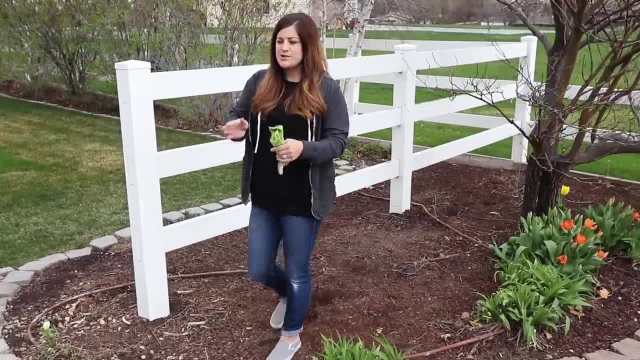 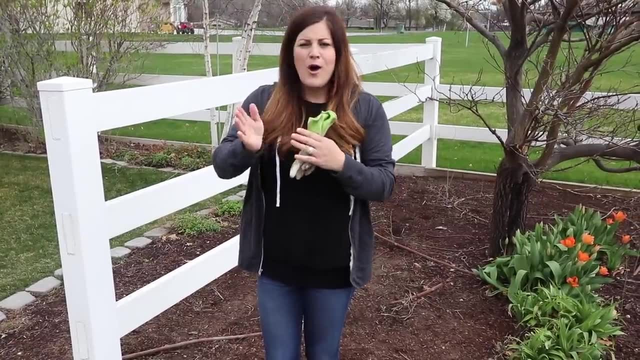 anything else. if you have a flower bed that you see from both sides, you do your tallest piece, usually in the center, and kind of go down on either side so that it kind of creates almost a a wall or a back in and of itself right through the center. so every area is a little bit different. 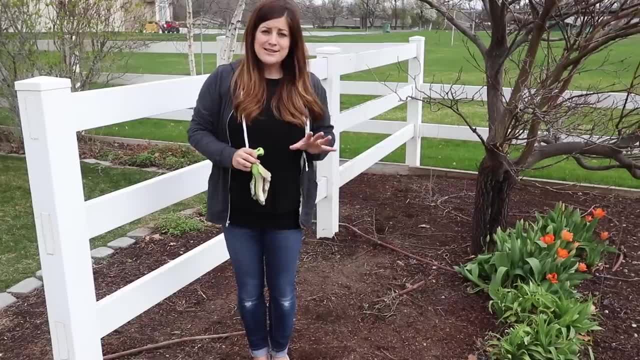 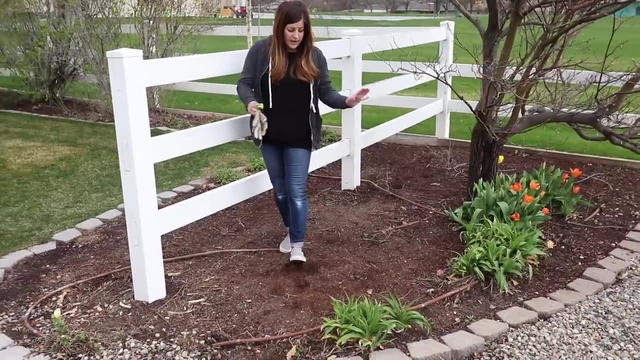 but those are five things that i always check for in every single area before i start, so let me explain what i'm going to do today. there's a couple of daylilies right here. i don't even know what variety they are. they were here when we moved in, and there's a hardy geranium there, so 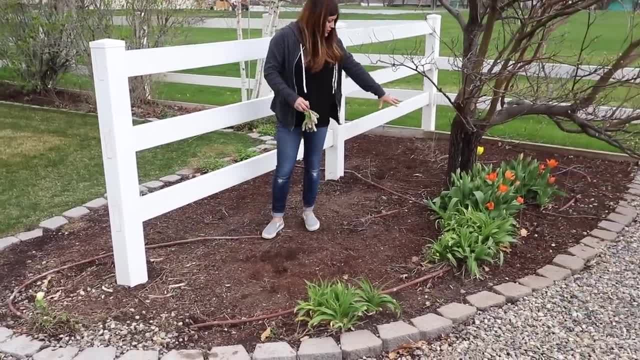 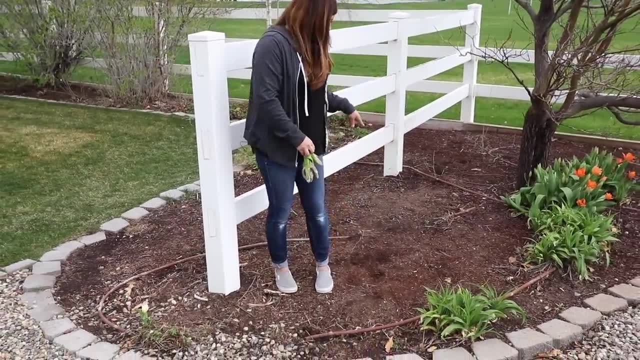 all three of those i'm going to dig out and then i'm going to leave all the tulips here and then, other than that, this whole area will be completely bare. then i'm going to come in with some irrigation and take care of that. before i place my plants, i want to make sure the water is on point. 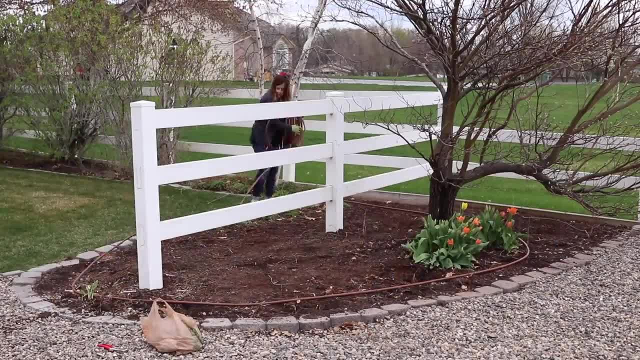 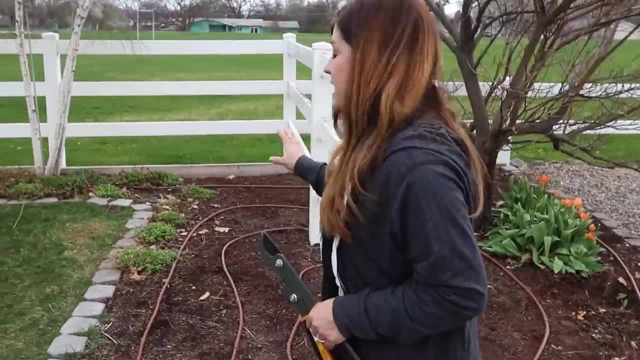 and make sure that everything is nice and dry, and so i'm going to take my plant so that it's looking a little trickier as it goes over the next few days. so let's get started, alright. so i've got all the drip tubing run, and what i ended up doing was 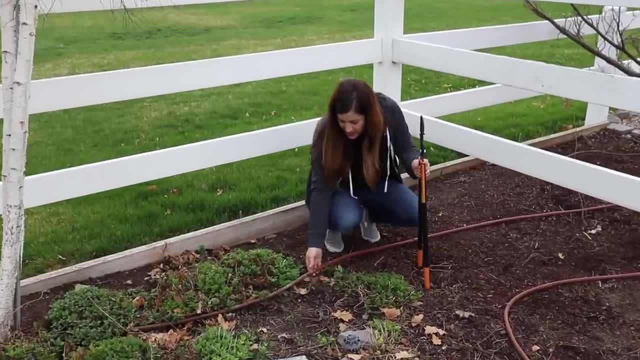 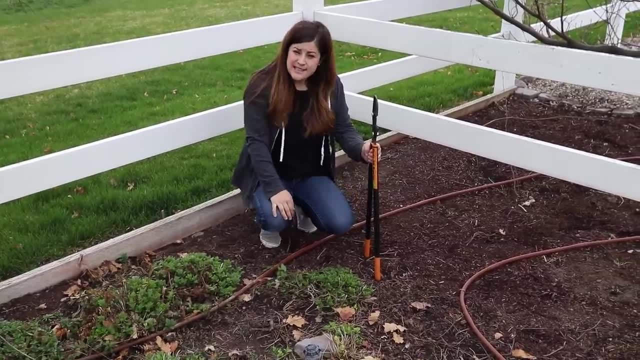 tearing all of the old stuff out and i just connected right here with my new stuff, so i cut all of the old existing stuff because it had hard water was plugging some of the emitters and it wasn't run very consistently so i just figured pulling. 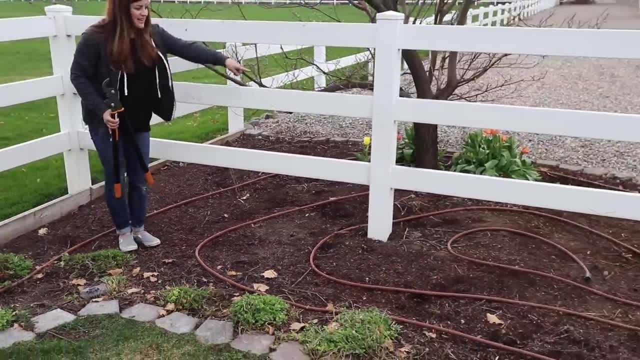 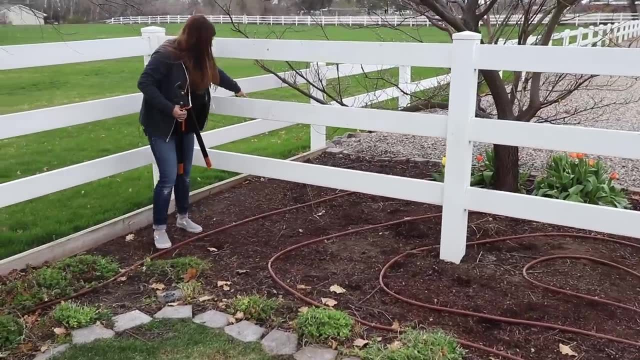 all of it out, and starting brand new is never a bad idea. wraps around in a circle until it ends right here, and it's actually kind of nice too, because I was able to not run any drip tubing over on this part right here because I don't want any weeds to grow. 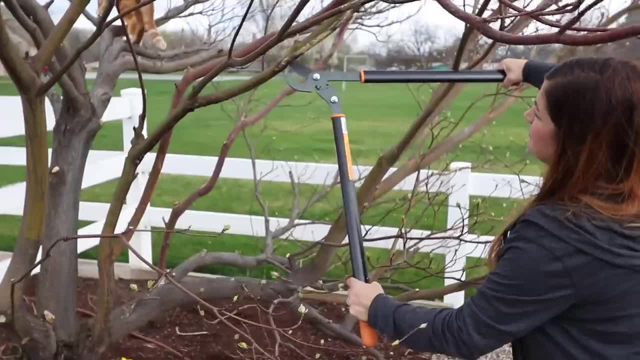 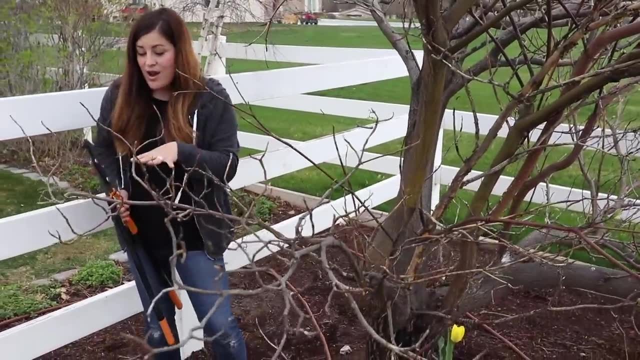 and once the tree leaves out, you can't even see this spot right here. The next thing I do need to do: I noticed that I have a couple of dead branches in here, so I'm going to clean this tree up and then I will place my plants and show you everything I'm going to put in this spot. So, by a couple, 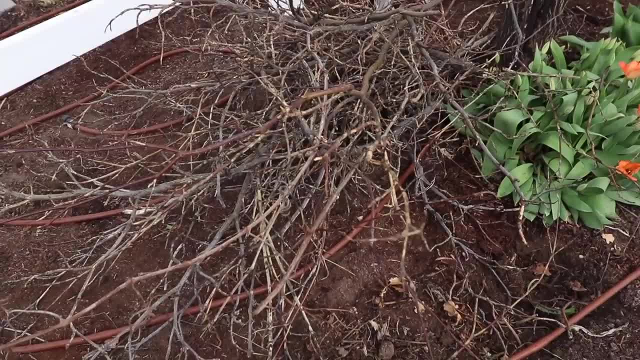 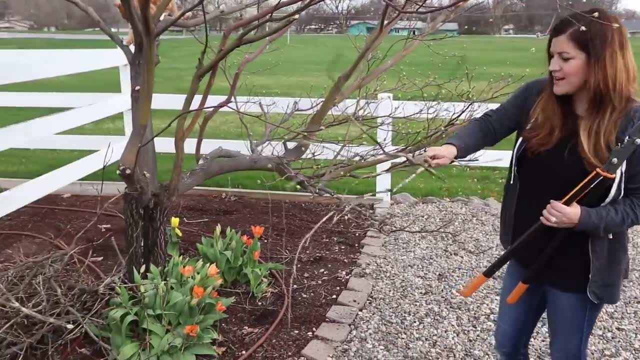 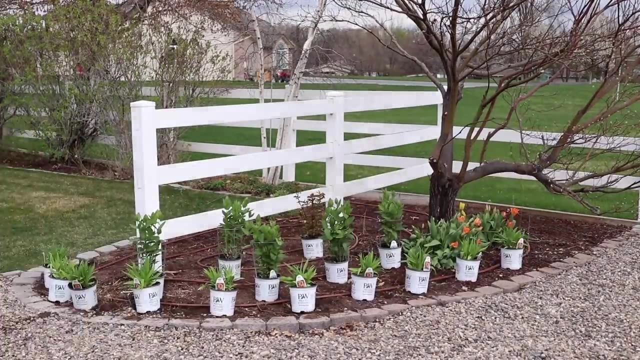 branches, I mean a whole pile. I got to looking at the tree and I really haven't done any maintenance on it in the past couple years, and this is what happens. So I'm going to haul all of this away and then I'm going to place all my plants and show you what I've got. All right, guys. so I've got three. 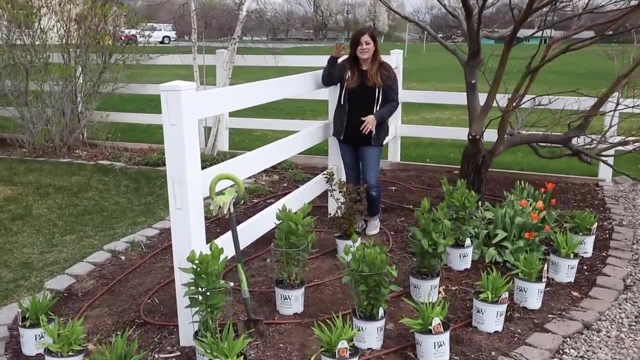 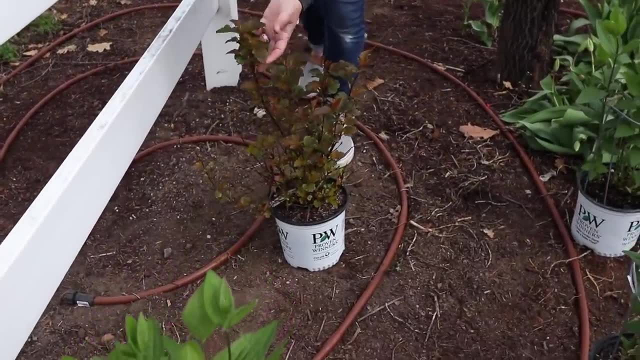 different kinds of plants in this area. so I'm going to start with my back layer first. This is my taller layer. This is called a gingerwine ninebark- Beautiful, beautiful bronze kind of orangey red color which is a great contrast to everything else that's going to be in this area. It grows about. 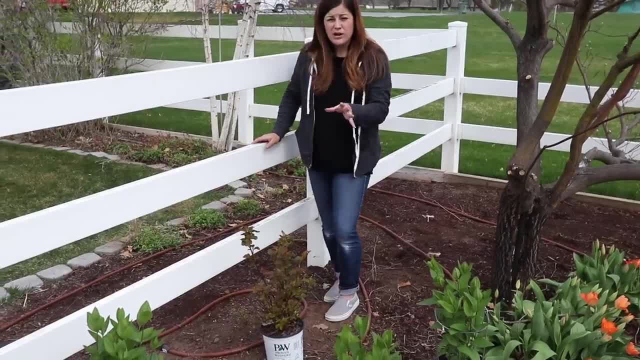 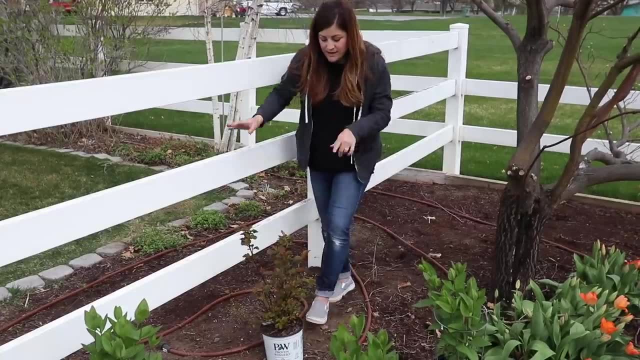 five to six feet tall and one and a half feet tall. So I'm going to put this in here and I'm going to back it up to this fence, because I want to utilize some of the color on the other side of the fence too, So some of the branches grow in between. that's even better, that's perfect. These are a. 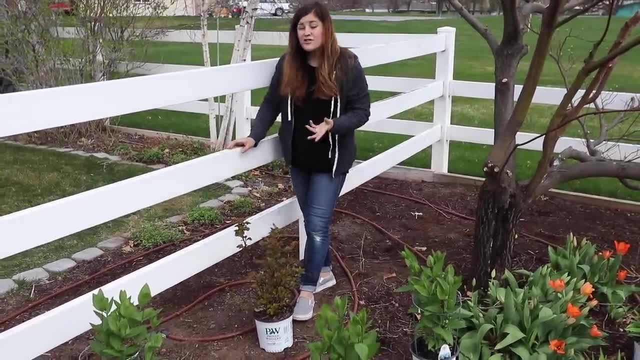 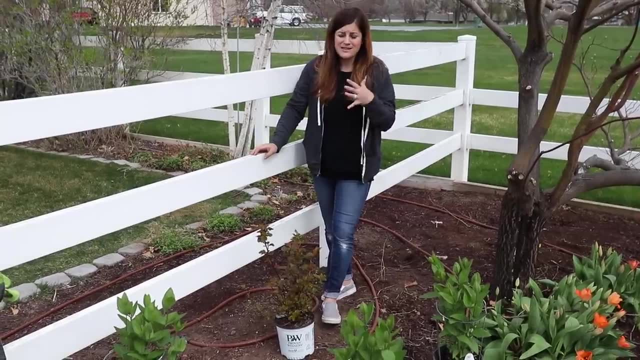 zone three through seven, so very winter hardy and they do bloom as well, like late spring through early summer White clusters of blooms that turn into red seed heads. so very pretty interest there and it also counts as winter interest because ninebarks get their name because of the peeling. 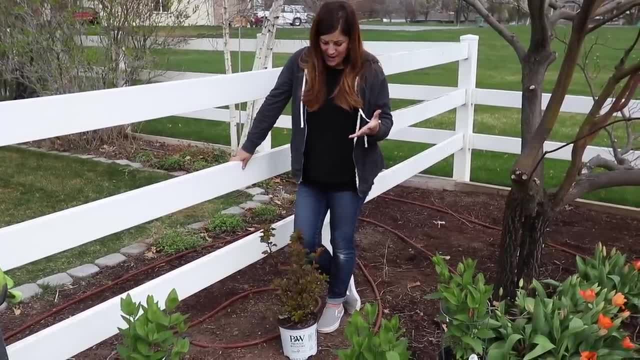 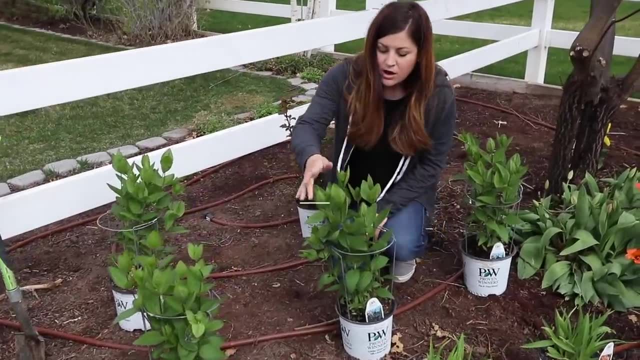 nature of their bark. Their bark is beautiful to look at in the winter time, So my next layer down is a really interesting plant. I'm so excited for you guys to see this. This is a new one this year called standby me clematis. It's a bush type clematis. instead of vining They grow. 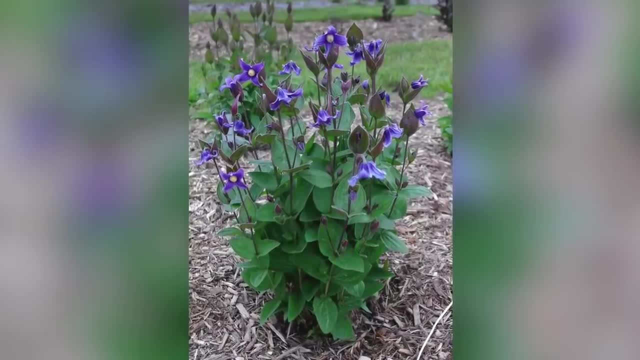 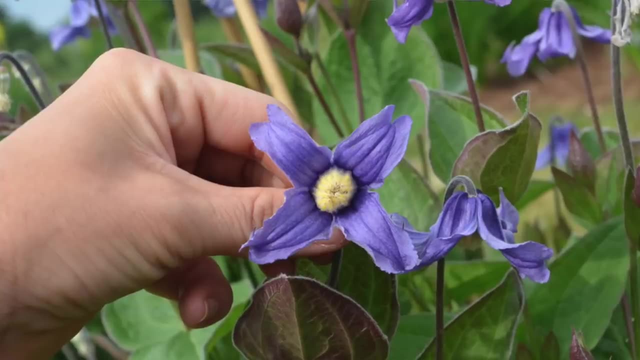 about three feet tall, two feet wide, so this will be a stair step down from my ninebark. They have the most gorgeous purple bell-shaped flowers and I think that that's going to be a really pretty color back here. Zone three through seven on these as well. so very, very winter hardy. Now you can see. 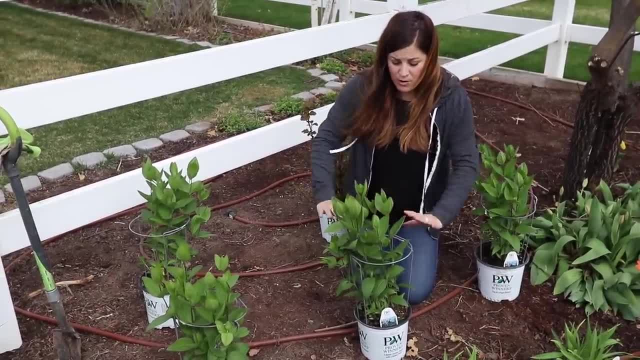 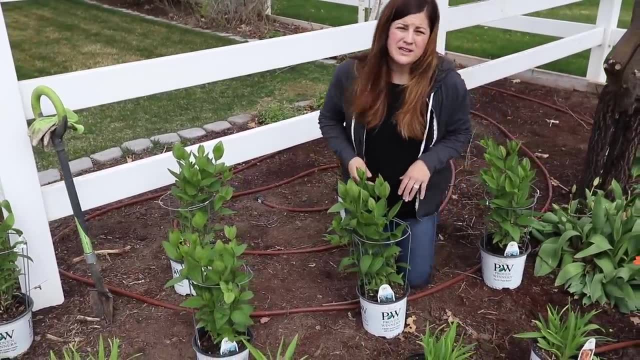 that I have a bunch of stakes, I should say, in the pot. so I'm going to leave those on or around these plants for this year and then I might graduate to a larger size ring next year to help support them. They do benefit from being supported, or once this area grows up and fills in, I can probably remove. 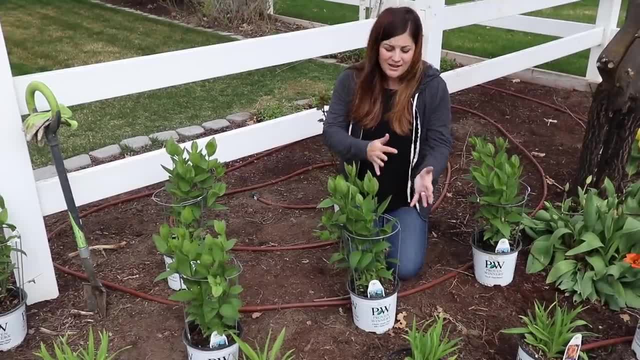 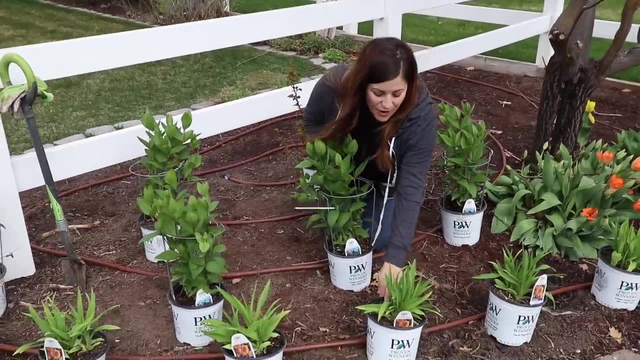 all supports, all together, because they'll support each other If they can kind of lean on each other a little bit, they don't need to be staked, but this first year, since they're all baby plants, I'm going to leave those on. The next layer down are orange smoothie daylilies and I put a bunch over here. 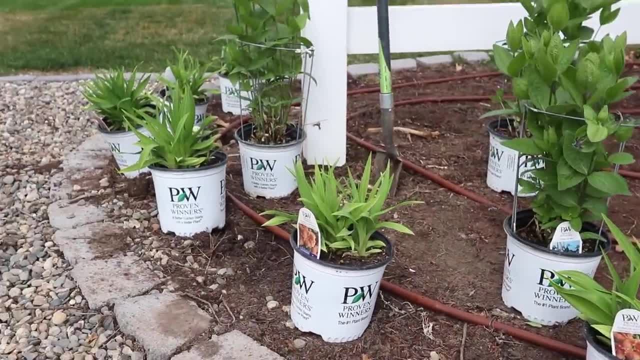 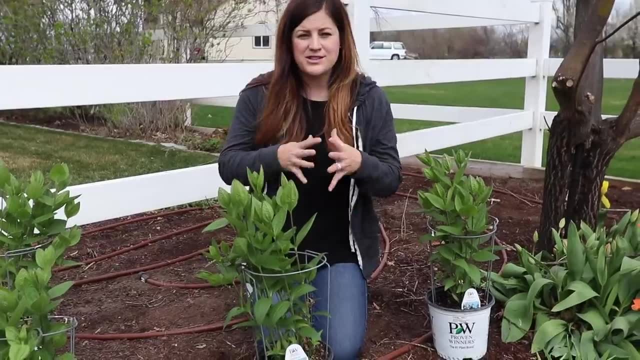 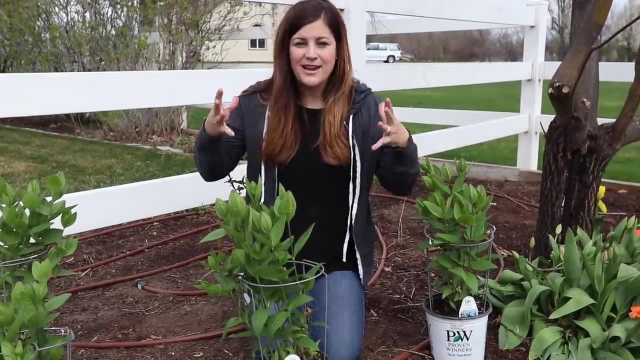 because I really wanted to make a statement and that's another thing I wanted to talk to you about. When you use too many different varieties of plants in an area, it can really be distracting. so it's a good idea to pick just a few varieties- maybe two, three, four, maybe at max- and just mass plant them so that it just is a striking. 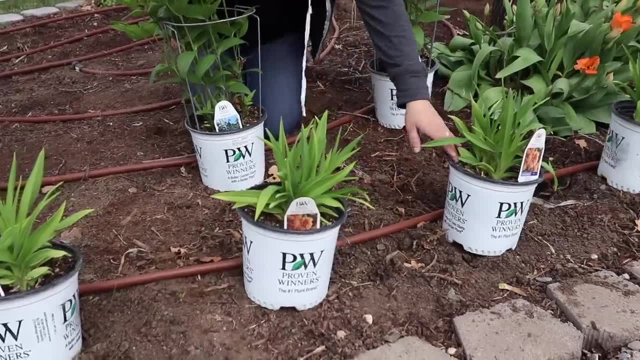 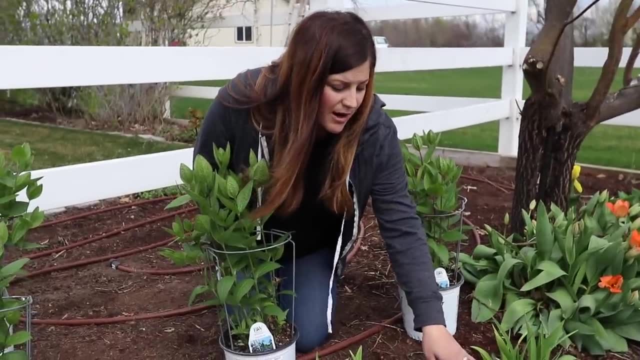 effect. So I've got, I don't know, nine or ten daylilies here that bloom mid-summer and then they re-bloom later on in the season, kind of a peachy orange bloom, and these grow about 20 to 24 inches tall. so this will be another. 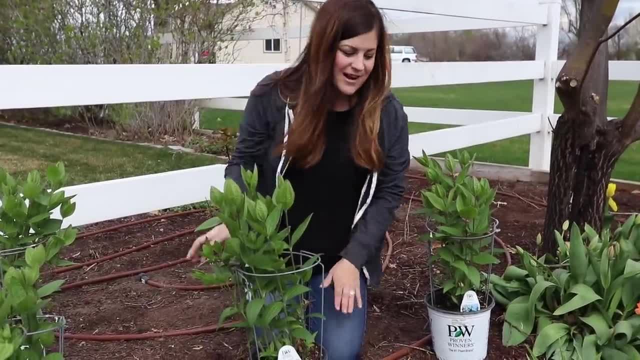 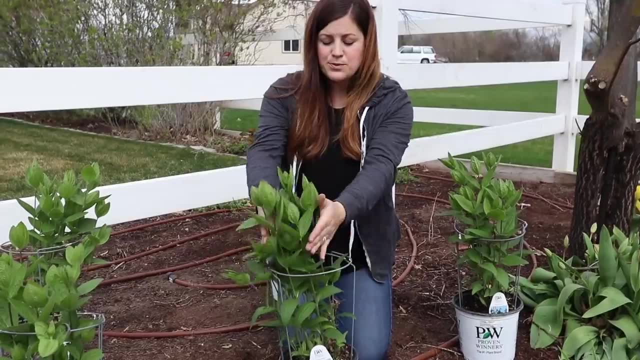 stair step down from the clematis, so I should have a very nice layered effect in this area. Both of these plants attract hummingbirds and their bloom times are a little bit staggered. so this one blooms late spring through mid-summer. this one blooms mid-summer and then again later in the season. so 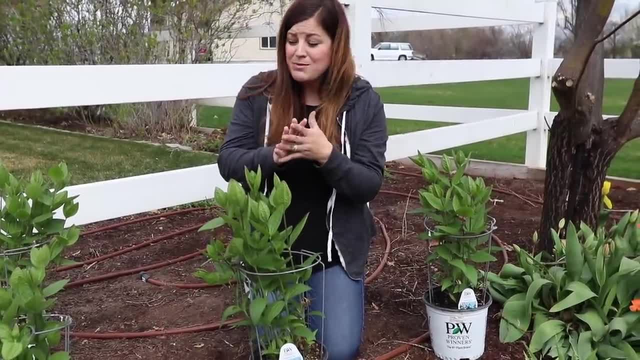 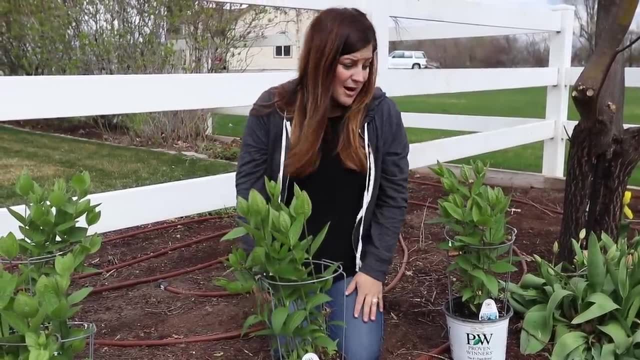 there should be a time, like a short window, where they're blooming together and it should be beautiful. but I'm glad that they have different bloom seasons because it'll be beautiful all all summer long. I'm really excited about this area, so I'm just going to get these all in the ground.